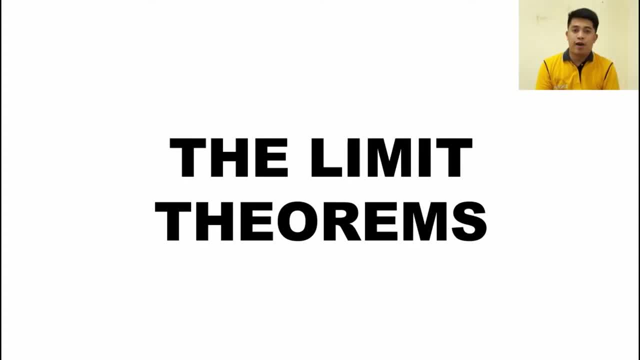 Welcome to another video, and for today we will be learning about the limit theorems. At the end of this lesson, the learners shall have illustrated the limit theorems and applied them in solving for the limit of algebraic functions. Mastering the limit theorems is a very big help for students in solving for the limit of functions. 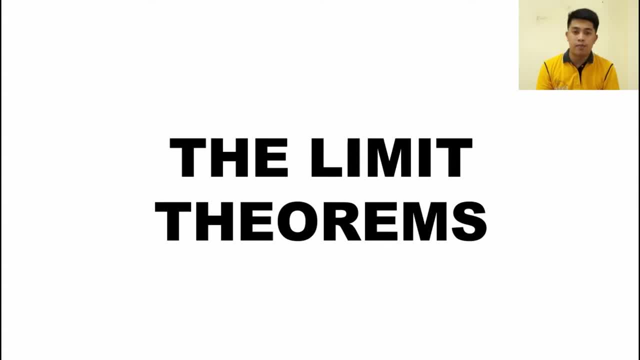 without doing the tedious process of making the table of values and illustrating the graph of the function. In this lesson we will be learning the limit theorems and apply them in solving for the limit of algebraic functions. The first theorem is called the limit of a constant. 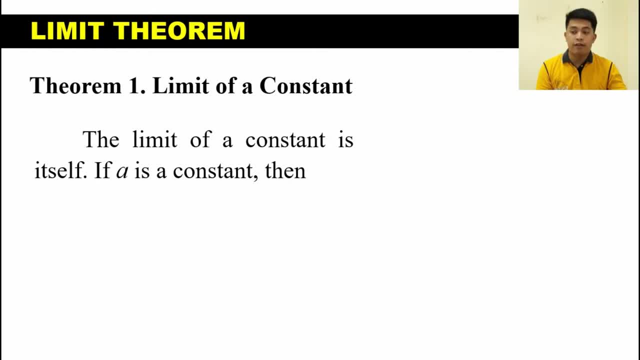 This states that the limit of a constant is itself. If a is a constant, then the limit of a as x approaches c is equal to a. Say, for example, we have a The limit, or we are asked to solve for the limit of: 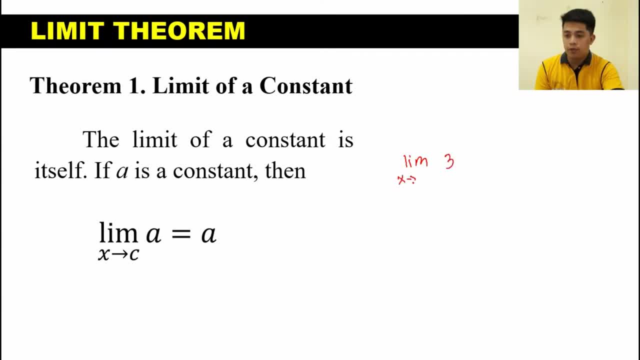 3 as x approaches 2, the answer is 3.. Another example: the limit of 1000 as x approaches 0 is equal to 1000.. Another example is the limit of pi. The limit of pi as x approaches 1, half is equal to pi, since pi is considered a constant value. 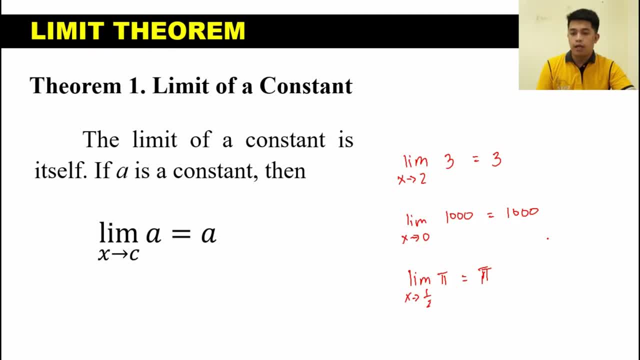 It has a value of 3.1416 and it is not a variable. Therefore, the limit of pi is itself. Okay, let's move on to another theorem, and it's called the limit of an identity function. This theorem states that the limit of a function, f of x equals 10.. 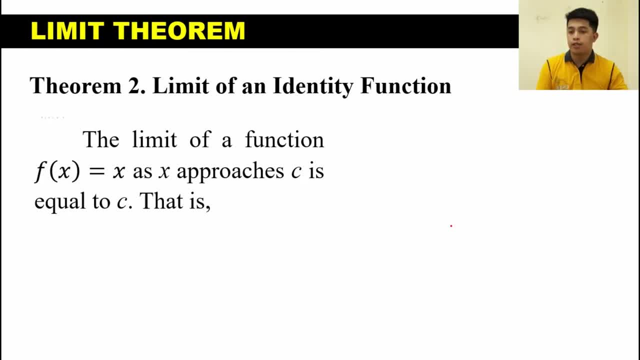 Therefore, the limit of a function f of x as x approaches c is equal to c. That is in symbols. we have the limit of x as x approaches c equals c. Say, for example, we have the limit of x as x approaches 0.. 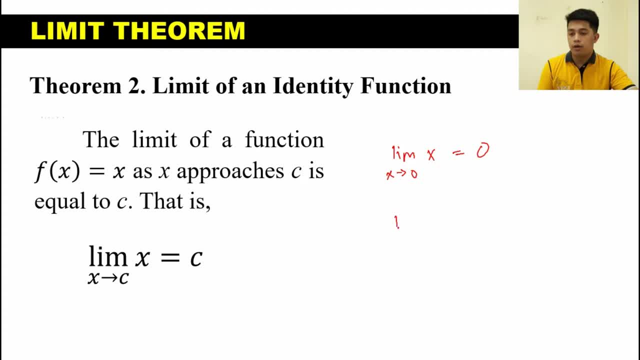 The answer is 0.. Another: the limit of x as x approaches 1 half is equal to 1 half. Another: the limit of x as x approaches 3 is equal to 3.. So if you are given an identity function, f of x equals x or y equals x. 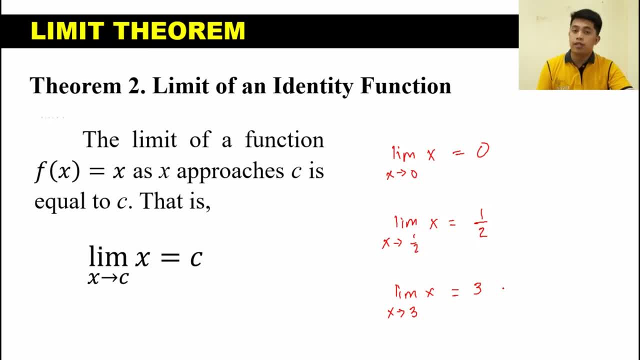 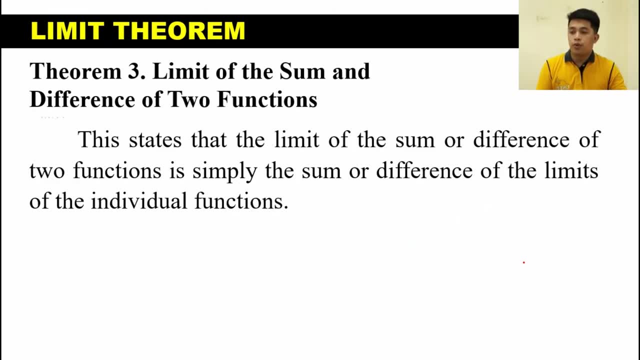 the limit of x as x approaches c is just equivalent to the value of c. Okay, Another theorem is called the limit of the sum and difference of two functions. This states that the limit of the sum or difference of two functions is simply the sum or difference. 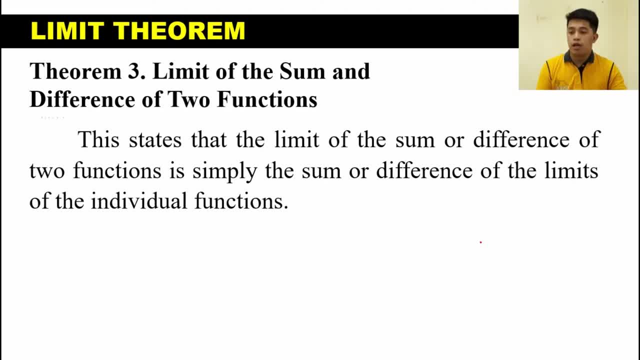 of the limits of the individual functions. For example, we are given: the limit of f of x as x approaches c equals l, and the limit of g of x as x approaches c equals m. Then the limit of the sum or difference of these two functions is denoted as the limit of f. 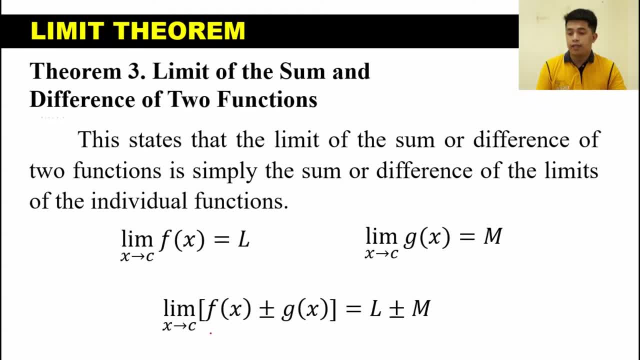 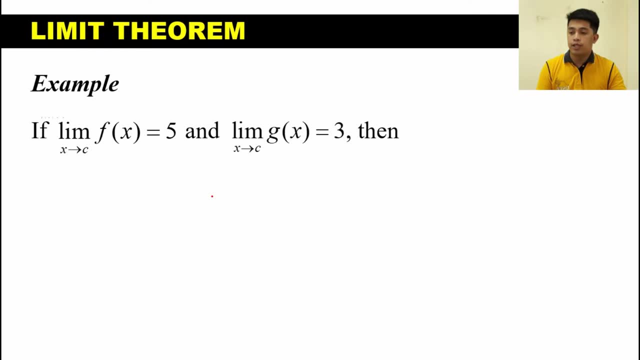 of x plus minus g of x as x approaches c equals l plus minus m. To illustrate this, let's have an example: If the limit of f of x as x approaches c equals 5 and the limit of g of x as x approaches c equals 3, then if we are asked to solve for the limit of f of x, 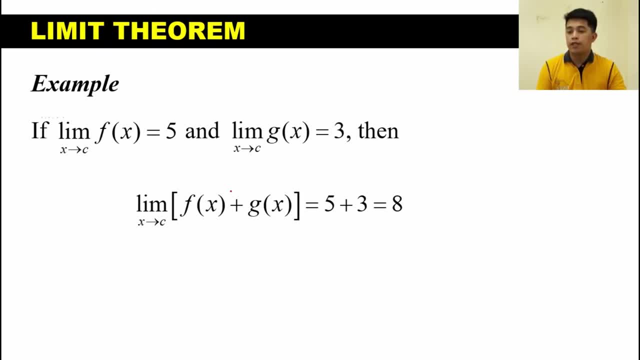 plus g of x as x approaches c equals 5, then the limit of f of x as x approaches c equals c. we just need to add the limit of the individual functions. So the limit of f of x is equal to 5.. The limit of g of x is equal to 3.. Since we already have the values of the individual, 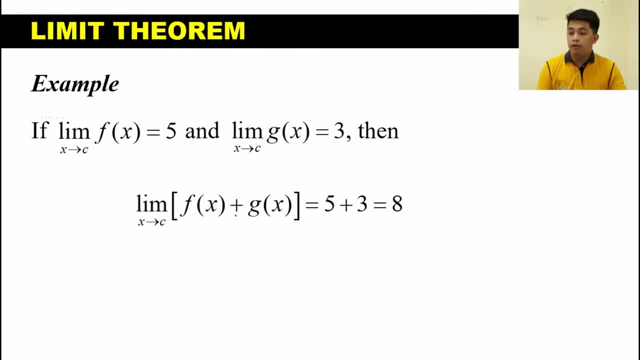 limits. if we are asked to solve for the sum of their limits, we just need to add them. So we have 5 plus 3 equals 8.. Therefore, the limit of quantity f of x plus g of x is equal to 5.. 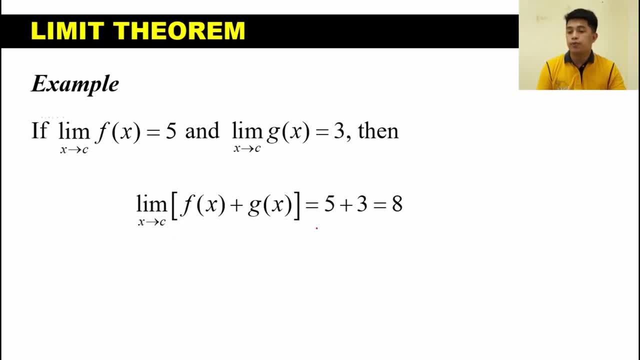 As x approaches c is equal to 8.. Another example is if we are asked to solve for the difference of the limits of these two functions. So we have here the limit of f of x minus g of x as x approaches c. Since we already have the values 5 and 3, we just have to subtract. 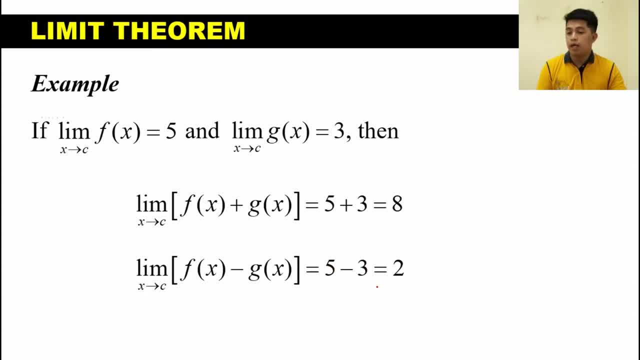 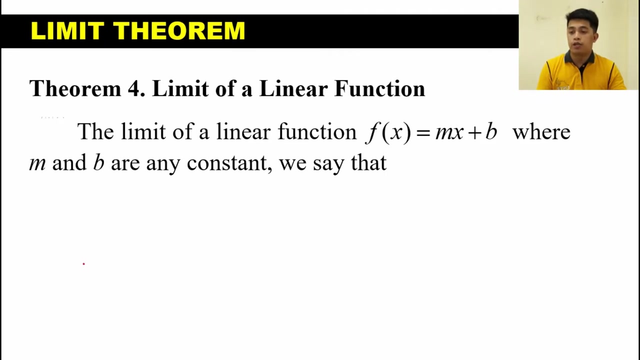 them We have: 5 minus 3 equals 2.. Therefore the limit of f of x minus g of x as x approaches c is equal to 2.. So that is the limit of the sum and difference of two functions. Another limit theorem is called the limit of a linear function. This states that the 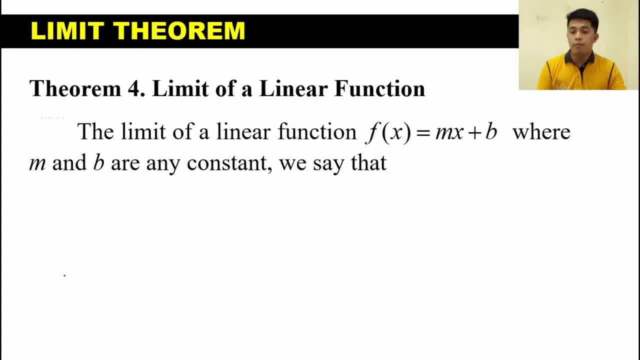 limit of a linear function, f of x equals m of x plus b. where m and b are n-constant, we say that the limit of m, x plus b as x approaches c is equal to m c. What happens in here is that m and b retains, since they. 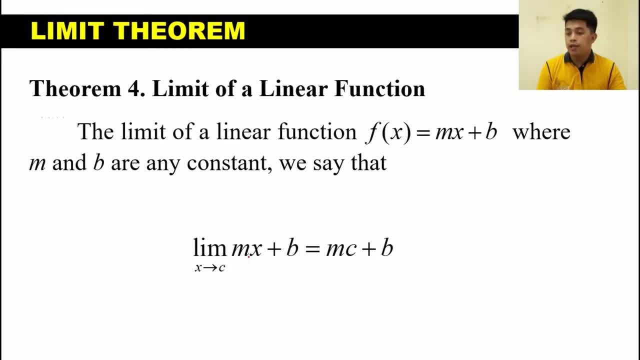 are constant values and the value of x in your function becomes c in your answer. Since, as what we had discussed in limit theorem, number 2, or in the limit of an identity function, the limit of x, as x approaches c, equals n, will remain constant. an end of the function. This means the society that works on an Madisonian. 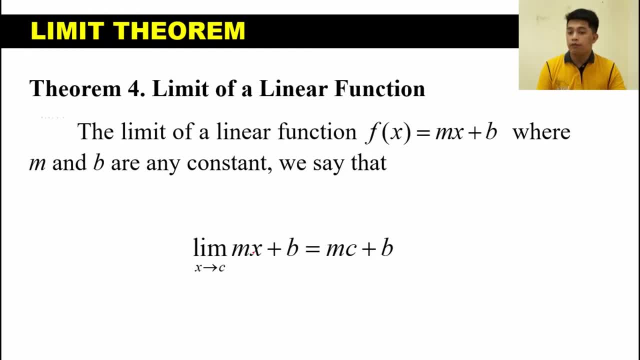 nós is thinking about developing a new model. So the system shall develop. n이라고 says a number which is no longer new, and it relies on the existence of functions by other people. So the systemравствуйте of the잖아요 temple is such that it's not efficient at all, because 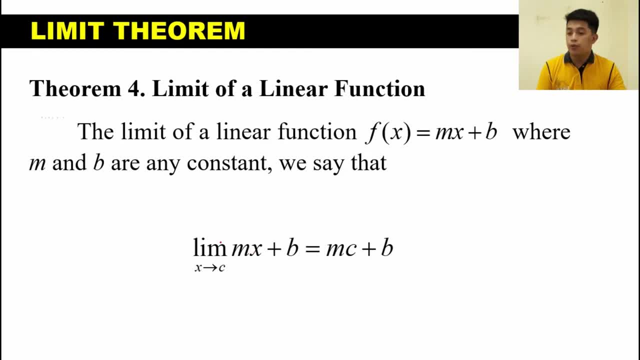 it will assume that everything is based on a function by every other being. that will be the same as ever. Therefore, this surprised here is being severe attention to the principle that c is equal to c. Therefore, the limit of mx plus b, as x approaches c, is equal to mc plus. 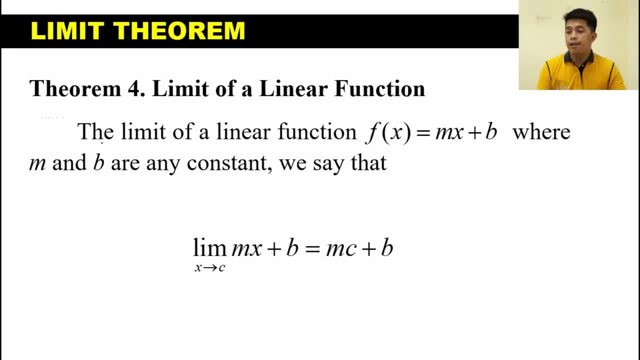 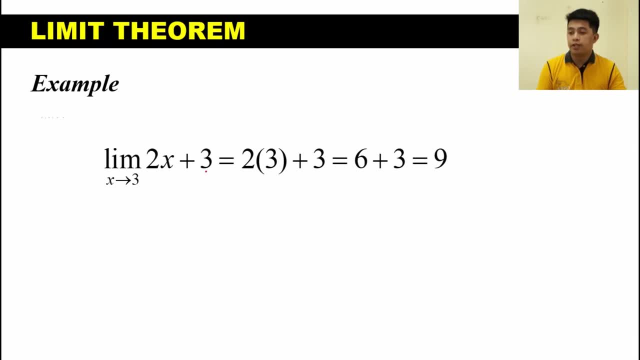 b. To understand this theorem, let's have an example. If we are asked to solve for the limit of 2x plus 3 as x approaches 3,, then what we need to do is to substitute 3 to the value of x, since the limit of x as x approaches c is equal to c. So we have here the constant. 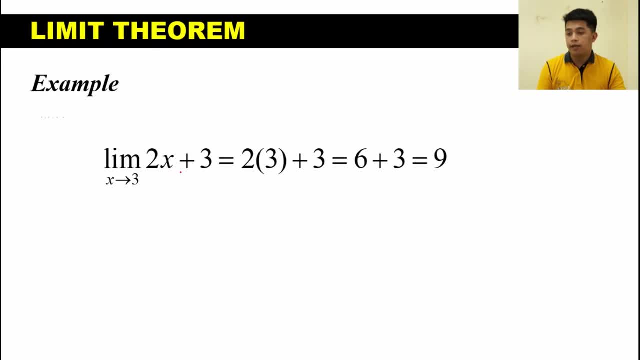 2 times the value of x or the value of c, which is the limit of x, as x approaches c. so 2 times 3, plus the limit of a constant is itself. so we have plus 3.. 2 times 3 equals. 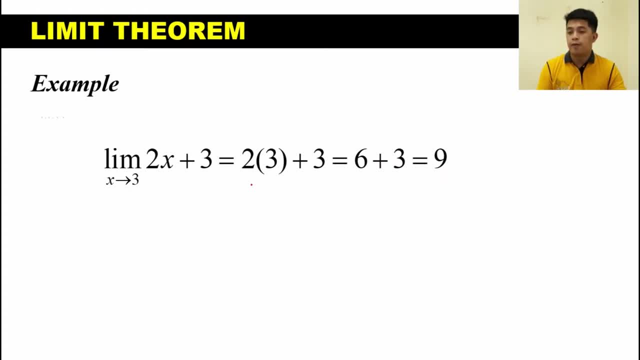 6, plus 3.. Therefore, the limit of 2x plus 3, as x approaches 3, is equal to 9.. This is simply substitution. Alright, this is one method that we have discussed in our previous video, which is the substitution. 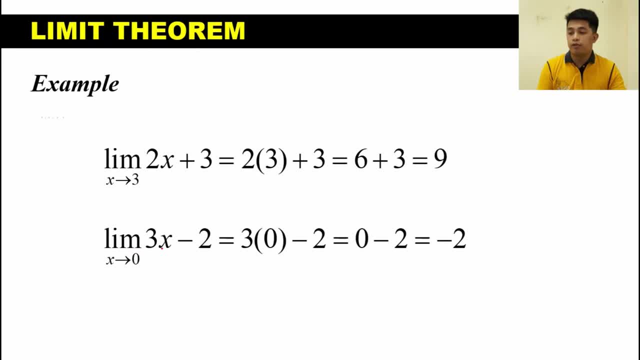 Another example: if we are asked to solve for the limit of 3x minus 2 as x approaches 0. We just need to substitute 0 to the value of x, So we have 3 times 0 minus 2 equals 0 minus 2 equals negative 2.. Therefore, the limit of 3x minus 2 as x approaches 0 is equal. 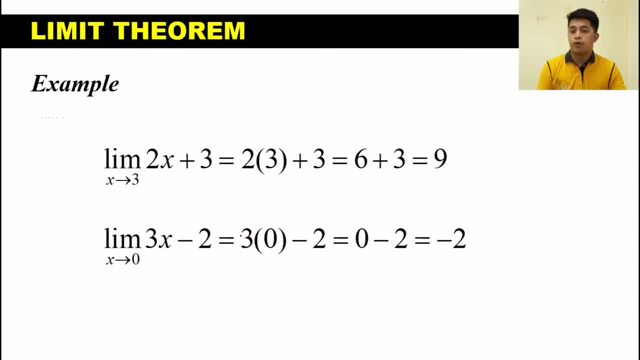 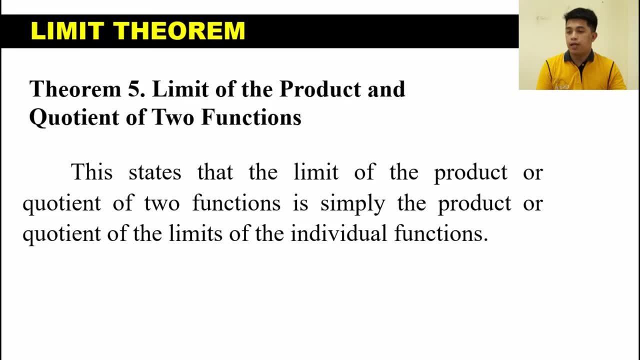 to negative 2.. So that is our theorem number 4.. Let's now move on to another theorem, and that is called the limit- theorem number 5. The limit of the product and quotient of two functions. This states that the limit of a product or quotient of two functions is simply the product. 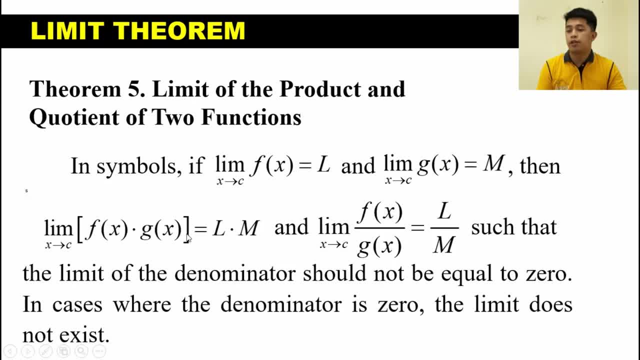 or quotient of the limits of the individual functions. In symbols we say that if the limit of f as x approaches c equals L and the limit of g as x approaches c equals M, then the limit of f times g as x approaches c. 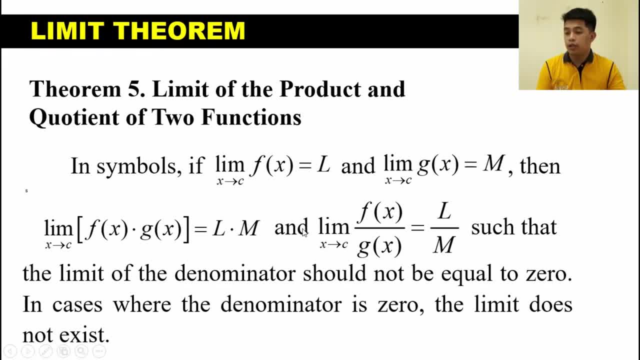 is equal to the product of their individual limits, L and M. So L times M, And the limit of f of x over g of x as x approaches c, is just equal to the quotient of the limit of the individual functions. So we have L divided by M or L over M, such that the limit of 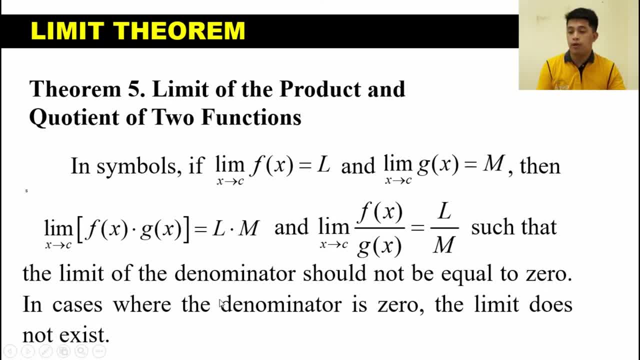 the denominator should not be equal to 0.. In case of the denominator, the limit of the denominator should not be equal to 0.. In case of the denominator, the limit of the denominator should not be equal to 0.. In cases where the denominator is 0,, the limit does not exist. 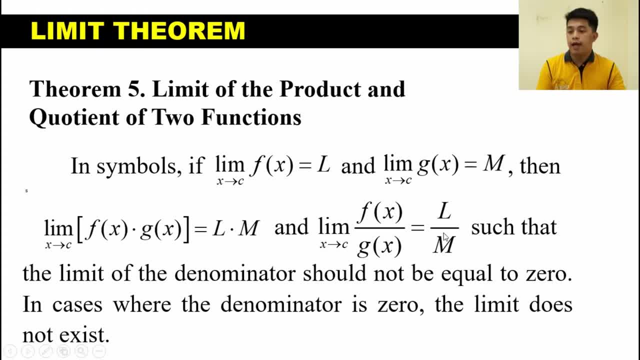 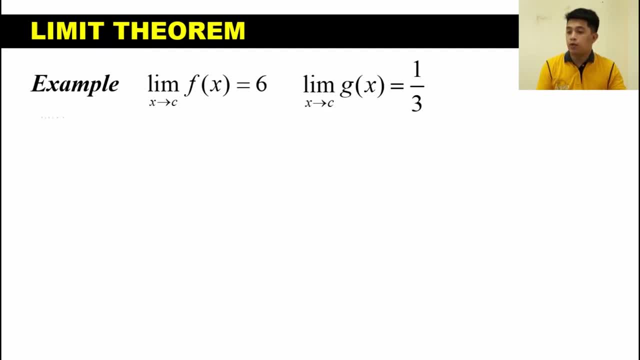 So to understand this theorem, let us have a simple example. The limit of f of x as x approaches c is equal to 6, and the limit of g of x as x approaches c is equal to 1 third. So if we are asked to solve for the limit of the product of f of x times g of 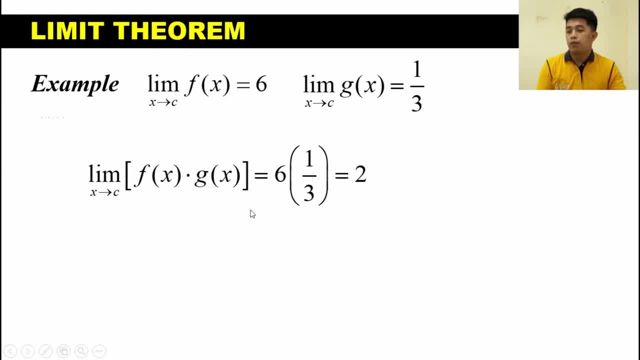 x. as x approaches c, we just have to multiply their individual limits 6 and 1 third. So we have 6 times 1 third. 6 times 1 is 6, 1 times 3 is 3.. 6 divided by 3 is 2.. Therefore, 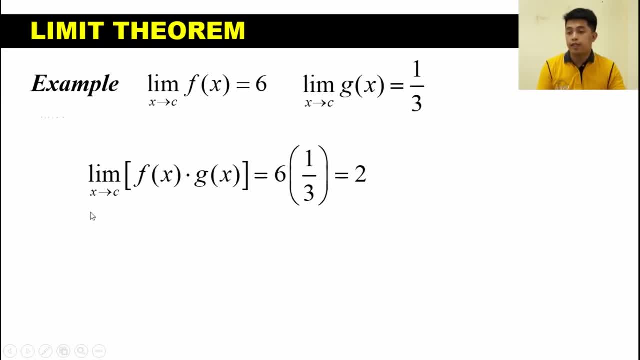 the limit of the quantity f of x times g of x as x approaches c is equal to 2.. How about quotient of the two functions We have? the limit of f of x over g of x as x approaches c equals the quotient of the limit of the individual functions. So we have 6 over 1 third Now, since. 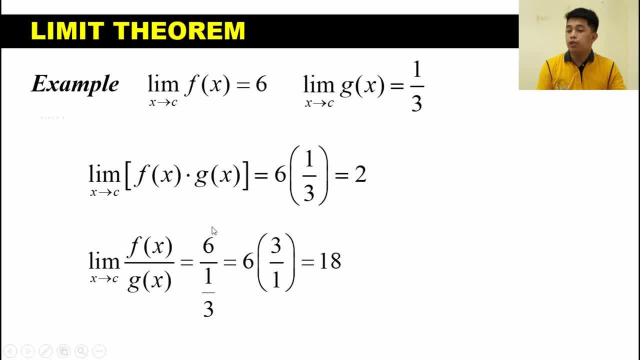 our denominator is a fraction. we multiply our numerator to the reciprocal of the denominator, So we have 6 times the reciprocal of 1, third, which is 3 over 1.. 6 times 3 is 18. divided by 1 is 18.. Therefore, the limit of f of x over g of x as x approaches c, is equal to 18.. 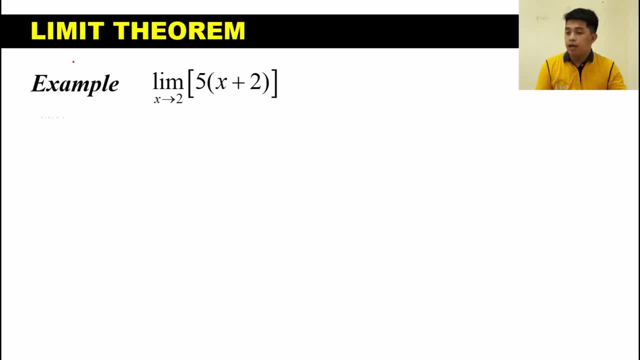 Now, what if the individual limits are not given? So, for example, we have the limit of 5 times the quantity x. What we need to do is to identify our individual functions. So we have here 5 as our f of x and x. 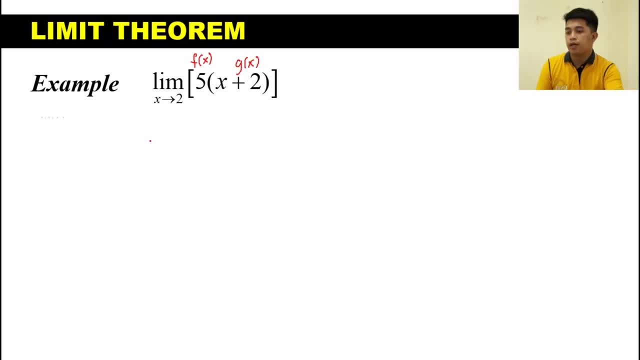 plus 2 as our g of x. So according to limit theorem number 5, the limit of the product of two functions is just equal to the product of their individual limits. So we can have the limit of 5 as x approaches 2 times the limit of x plus 2 as x approaches 2.. 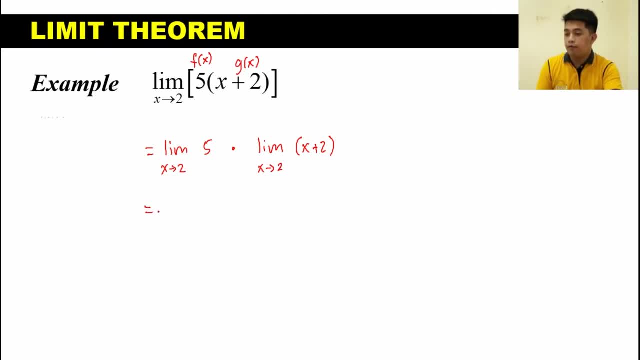 Now solving for the limit of the individual functions. we have here the limit of a constant. Now, what do we know about the limit of a constant? According to theorem number 1,, the limit of a constant is its self. So the limit of 5 as x approaches 2 is just equal to 5 times the limit of x plus 2 as x. 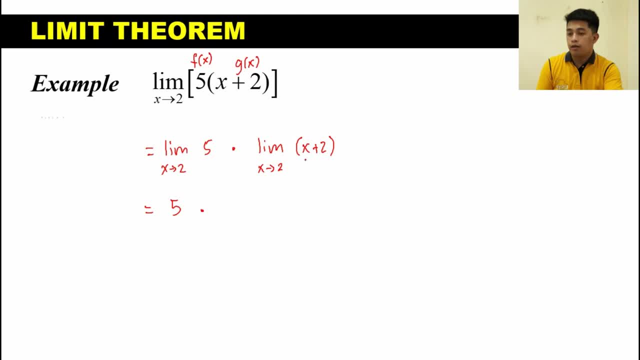 approaches 2.. And this is a function in the form mx plus b, where m is equal to 1. So we can just substitute 2 to the value of x. We have 2 plus 2. The answer is 4.. So 5 times 4 equals. 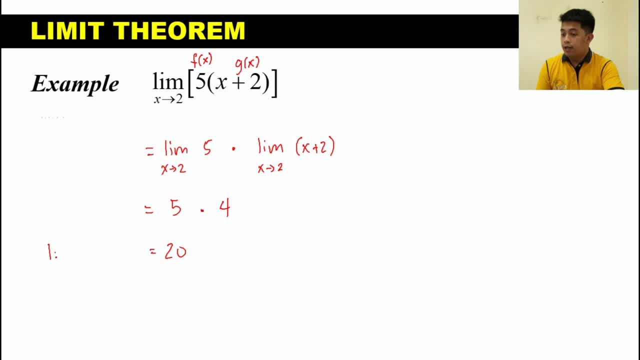 20.. Therefore, the limit of 5 times x plus 2, as x approaches 2, is equal to 20.. Now what if we use distribution before we evaluate the limit? Say, for example: in this case we have the limit of 5 times x plus 2, as x approaches 2.. But if we distribute 5 first, this will become: 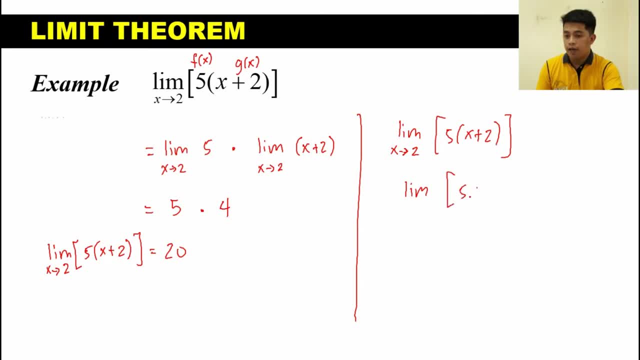 the limit of 5x plus 10 as x approaches 2.. Now, if we solve for the limit of this one, this will become 5 times 2, which is 10 plus 10 equals 20. therefore, the limit is 20 and the answer is just the same. 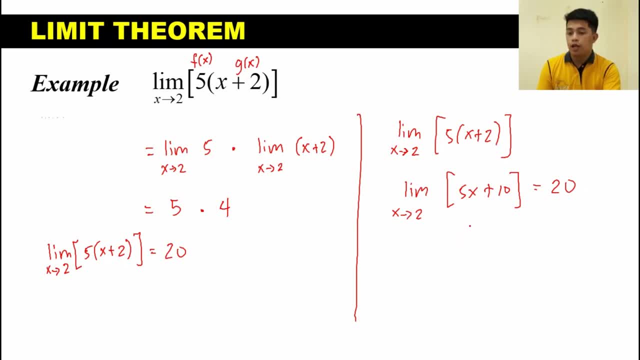 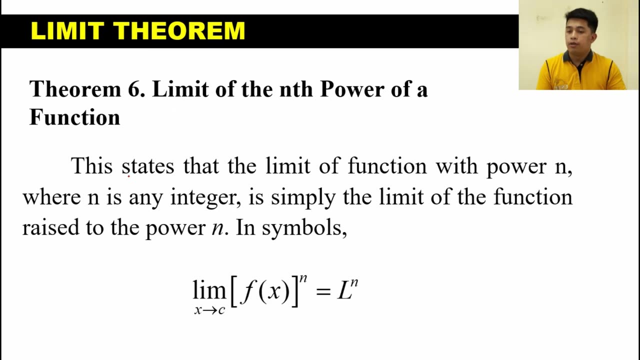 so whatever process you follow, as long as you make sure that your process is correct, then you will get the same answer. now let's move on to another limit theorem, and that is called the limit of the nth power of a function. this states that the limit of a function with our n, where n is any. 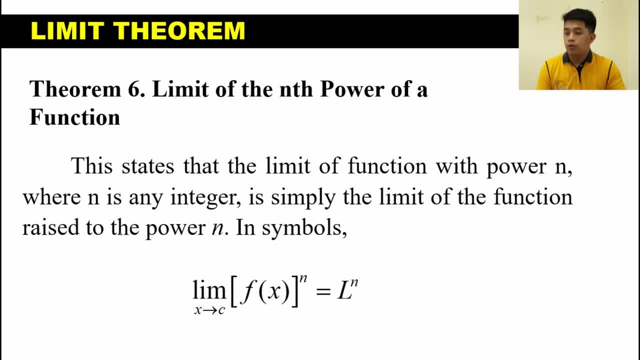 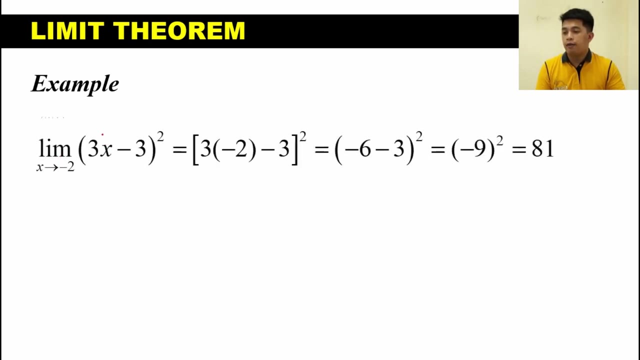 integer is simply the limit of the function raised to the power of n. in symbols, we have the limit of f of x raised to the power of n. as x approaches, c is equal to l to the n. to understand this one, let's have a simple example. what if we have the limit of 3x minus 3 squared as x approaches? 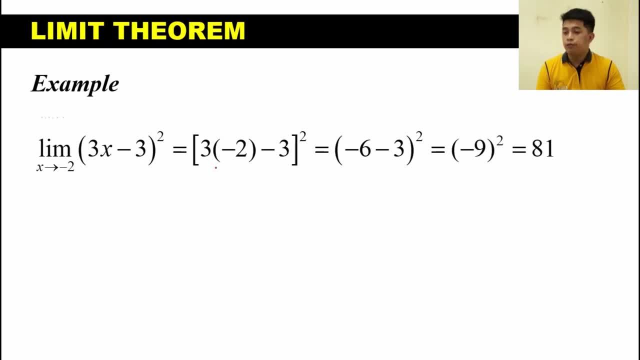 negative 2. what we need to do is to solve first the limit of f of x before we raise that one to the power n or the power 2. so solve for the function inside. we have 3 times negative 2 minus 3 raised to the power of 2. 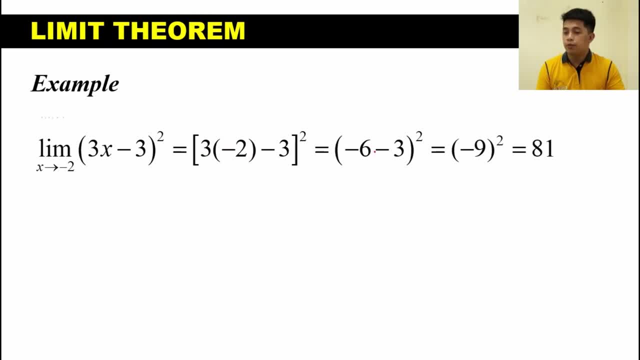 equals. we have 3 times negative. 2 is negative. 6 minus 3 raised to the power of 2 equals. simplify what's inside your parenthesis. we have negative. 6 minus 3 equals negative. 9 negative 9 squared is equal to 81. therefore, the limit of quantity: 3x minus 3 squared as x approaches negative 2 is: 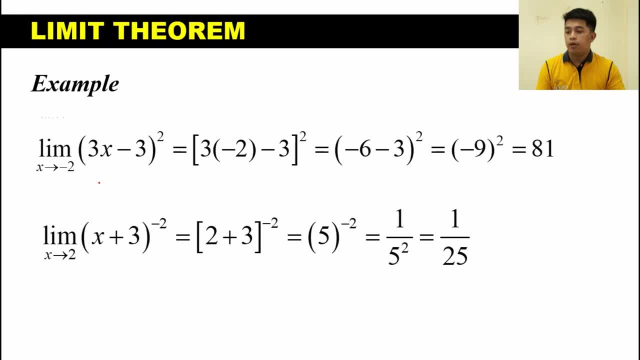 equal to 81. another example is the limit of quantity 3 raised to the power of negative 2. this is equal to three pp, 3 p, the power of negative 2. so 2 plus 3 is 5 raised to the power. 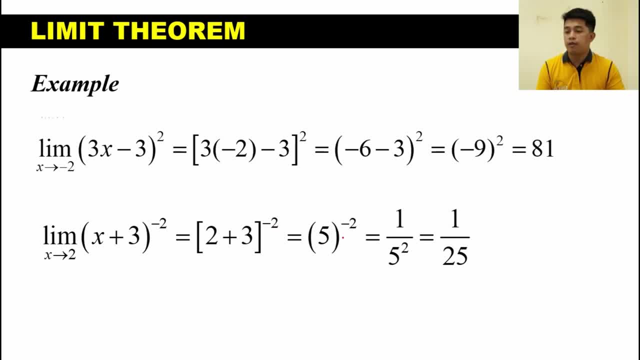 of negative 2, since the exponent is a negative exponent. so Playing with a, the picture is айте funny, i like. i now soda number. we can rewrite this one as 1 over 5, squared by the loss of exponent, Now 1 over 5. 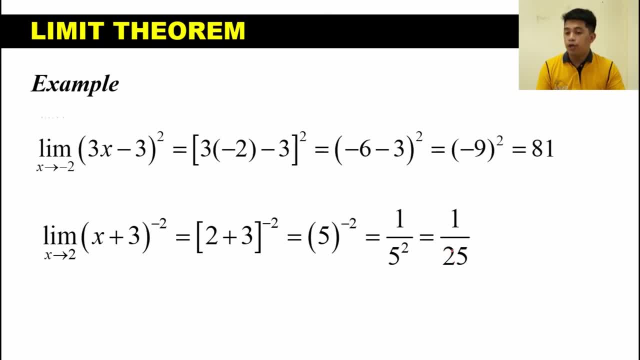 squared is simply 1 over 25.. Therefore, the limit of the quantity x plus 3 raised to the power of negative 2, as x approaches 2, is equal to 1 over 25.. Now let's move on to the last limit theorem. 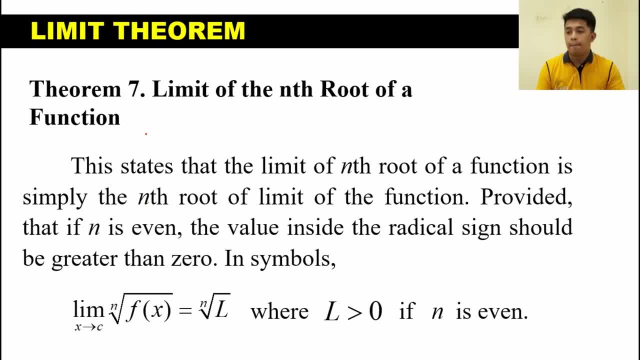 and that is called the limit of the nth root of a function. This states that the limit of the nth root of a function is simply the nth root of the limit of the function, provided that if n is even the value inside, the radical sign should be greater than 0.. 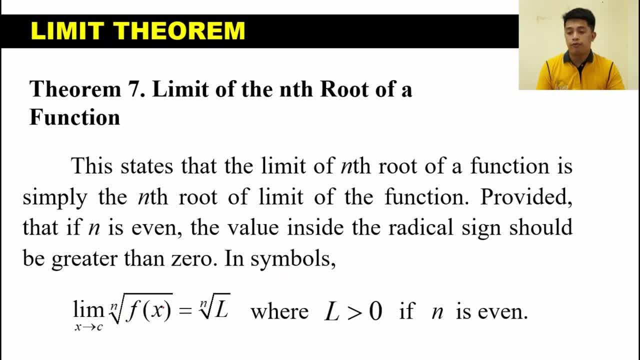 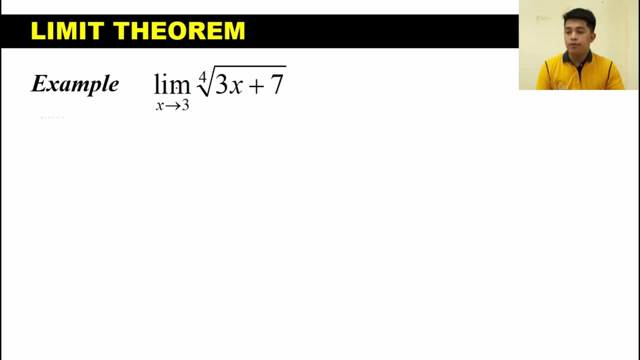 And so, symbols, we have the limit of the nth root of f, of x. as x approaches, c is equal to the nth root of l, where l is greater than 0, if n is even, For example, the limit of the fourth root of 3x plus. 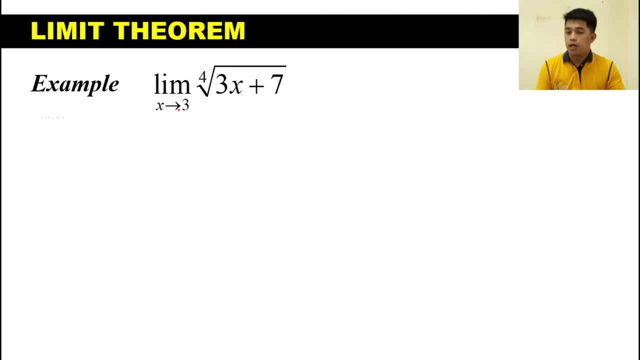 7 as x approaches 3.. We can simply substitute 3 to the function inside our radical sign, So we have the fourth root of 3 times 3 plus 7.. 3 times 3 is 9, so we have 9 plus 7.. So 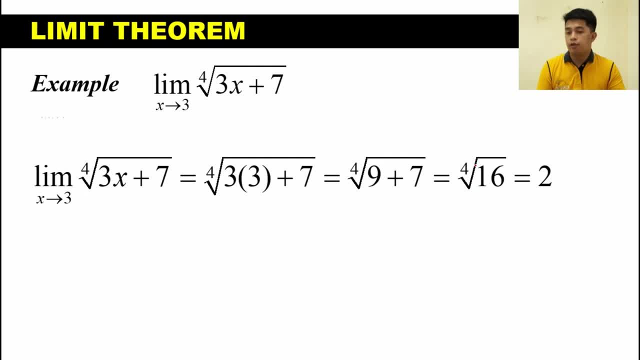 we have fourth root of 16, and the fourth root of 16 is equal to 2.. Notice that the value of our index is 4, which is even, and the value inside the radical is greater than 0. Therefore, the limit of the root of f is equal to 0. 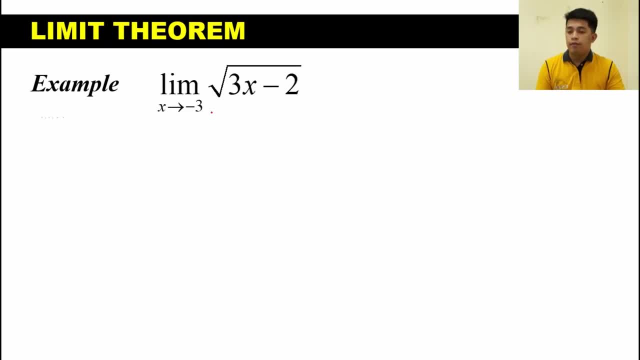 Therefore, the limit of the root of f is equal to 2.. limit exists and that is equal to 2.. Let's have another example: The limit of the square root of 3x minus 2, as x approaches negative 3.. So since the index is 2, we have an invisible 2 here. 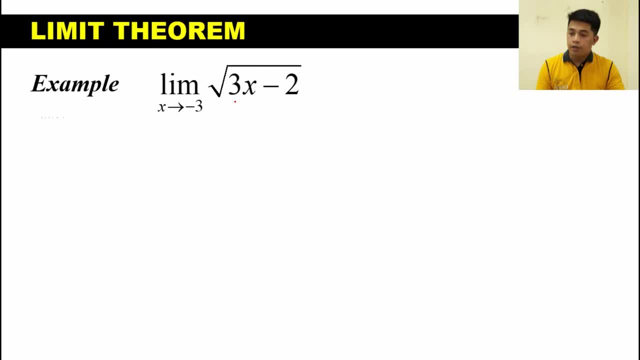 the limit of the inside function, which is 3x minus 2, should be greater than 0 since, according to theorem number 7, if your index is even the value of your radicand should be greater than 0.. Let's try to evaluate this one. We have the limit of the square root of 3x minus 2 as x approaches. 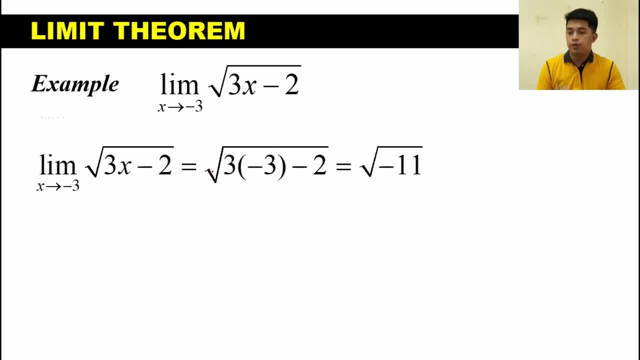 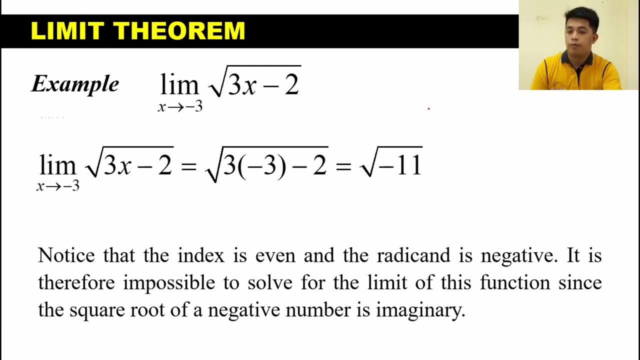 negative 3 is equal to the square root of 3 times negative 3 minus 2, which is equal to negative 11.. Now notice that the index is even and the radicand is negative. It is therefore impossible to solve for the limit of this function, since the square root of a negative number is imaginary. Therefore, 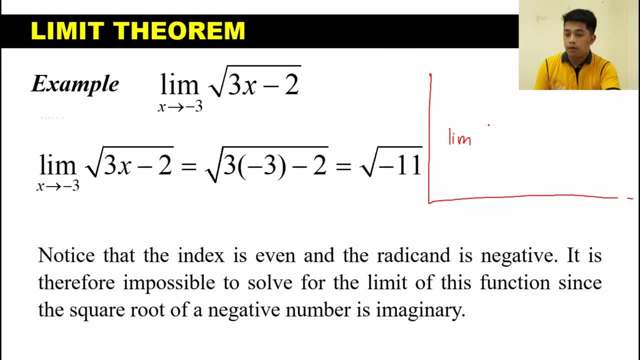 we can conclude that the limit of the square root of 3x minus 2, as x approaches negative 3, is equal to 0.. So let's have another example. We have the limit of the square root of 3x minus 2. 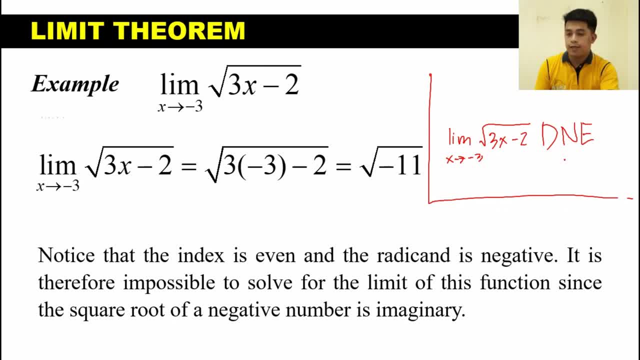 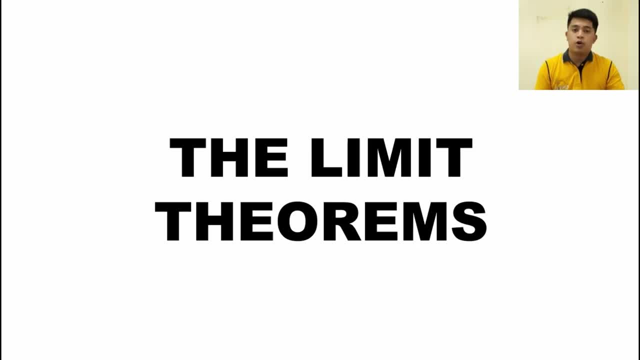 which is equal to 1 equals sign. Just put dn. So that ends our discussion about the limit theorems. I hope you have learned something in this video, So if you have questions or clarifications, just comment down And for.